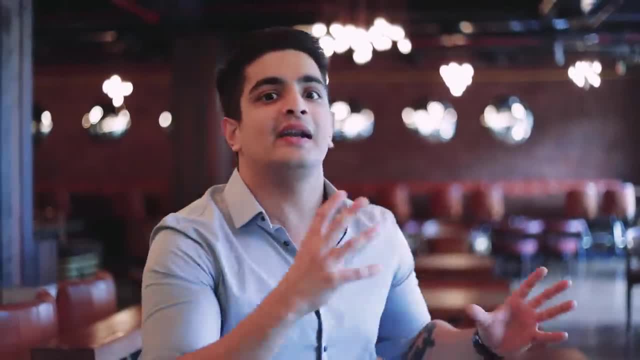 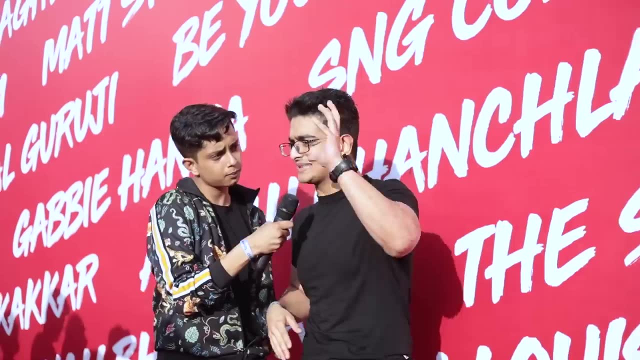 big weakness of mine. So for me to start my own Hindi channel was very difficult, But I used a few simple tricks to improve on my spoken Hindi, and I believe that those same tricks can be applied to English. As with any life skill. I believe that you've got to make the process easy for yourself. 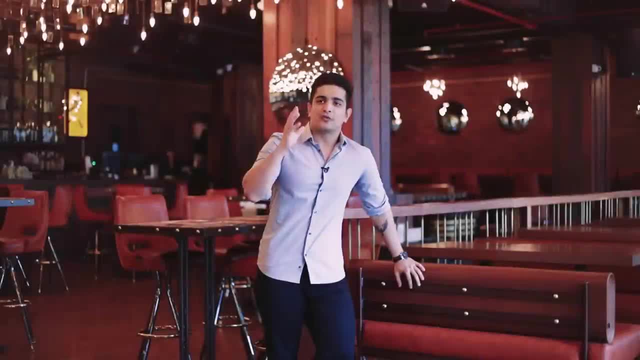 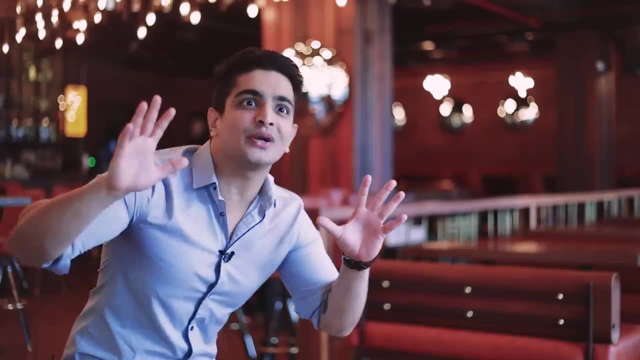 and your big brother got you covered. So if you ask most people what the first step is when it comes to improving a spoken language, they'll say: you start looking at the news, join classes, look at Shashi Tharoor. nope, I don't believe that that's true. I believe that if you want to learn a new language, 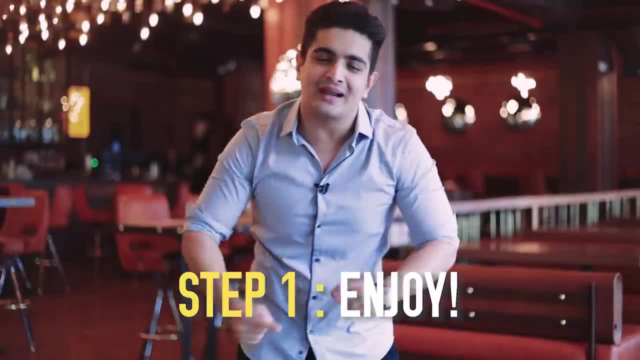 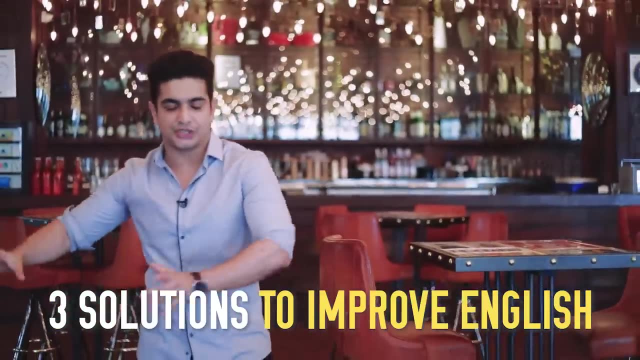 you've got to enjoy the process, And, keeping enjoyment in mind, I've got you three easy solutions. Okay, so these three solutions are basically three options in order to improve on your English. If you really want to improve it, you've got to make it a habit to practice these. 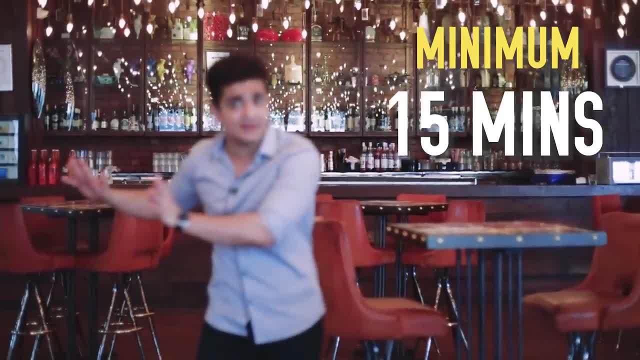 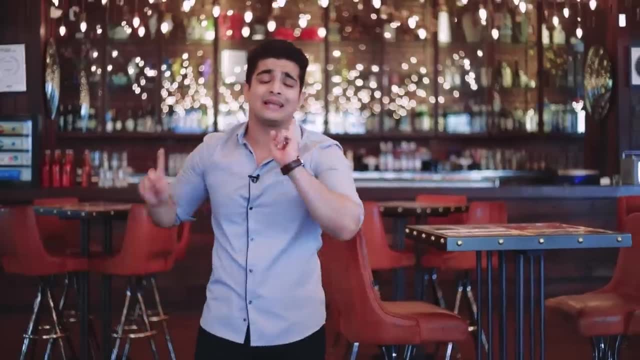 three options. You've got to practice it for a minimum of 15 minutes every day and for a maximum of however long you want. I'd suggest one hour a day is enough for you to practice. Good to start with Option number one: easy video content. We're talking cartoons primarily, where. 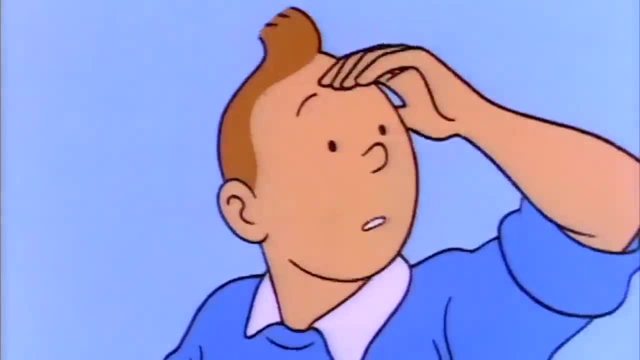 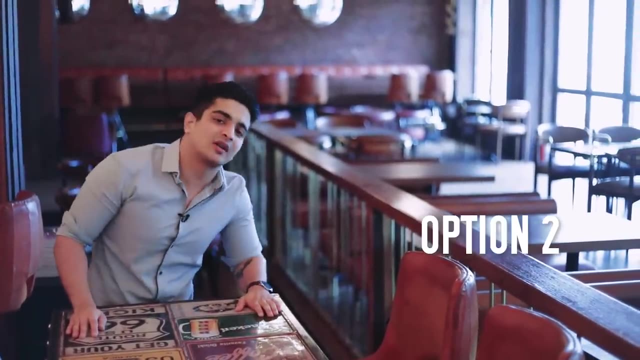 the language used is super simple. It's meant for children to understand. Easiest way to improve your English. And if you're one of those bros who thinks that you're too old to watch cartoons, that's okay. Your other options are to watch a lot of English video content. Maybe watch other 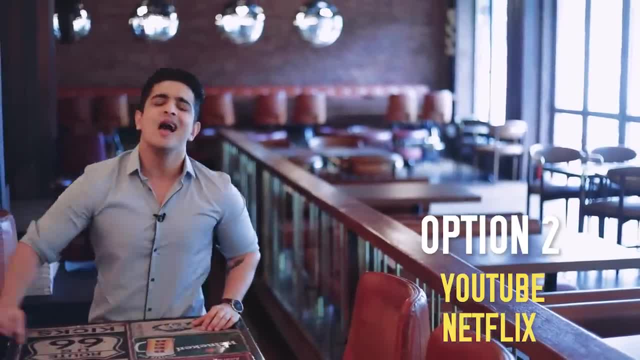 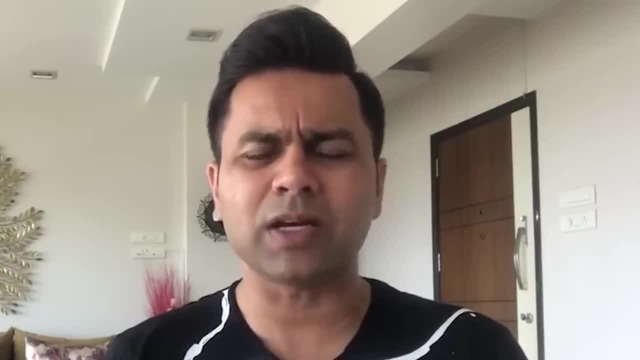 beer biceps videos. maybe watch other YouTube channels, watch Netflix Option. number three is my personal favorite. Akash Chopra helped me to improve my Hindi by his Hindi cricket commentary Chup kar. Akash Chopra. I suggest you go and watch English cricket commentary, especially Indians who are 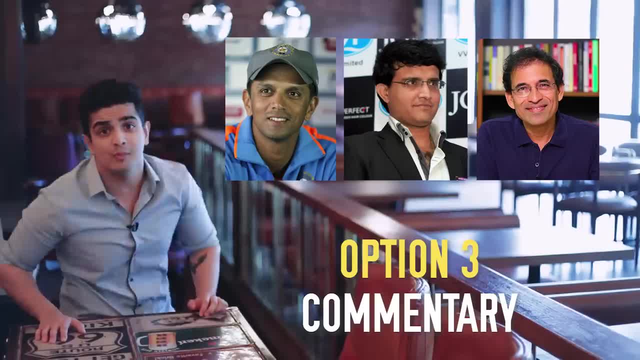 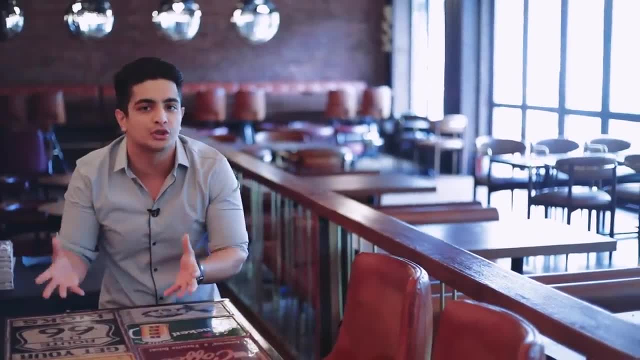 commentating in English. Think Rahul Dravid, Sourav Ganguly, Harsha Bhogle is fantastic. Go watch a lot of commentary. Basically, choose a piece of video content that you really enjoy watching and that'll do the trick for you. That'll help you improve on your English or your Hindi. 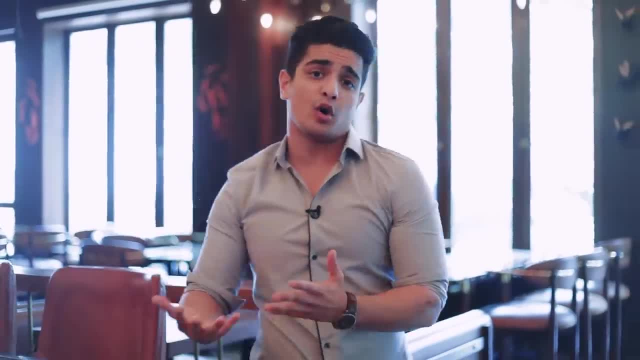 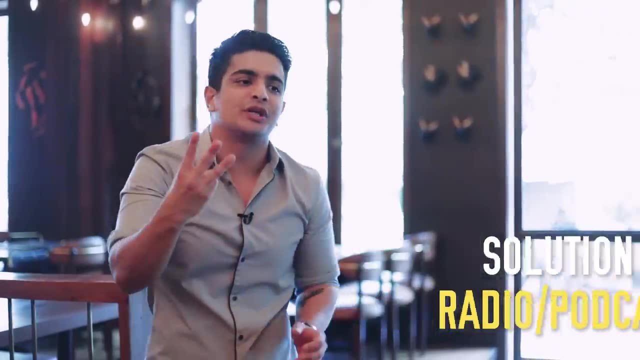 Also keep in mind that that's just the first solution: watching a lot of video content. If you're someone who doesn't enjoy video content, that's okay. If you enjoy listening to the radio or podcasts, do that. If you're someone who doesn't enjoy listening to the radio, do that. 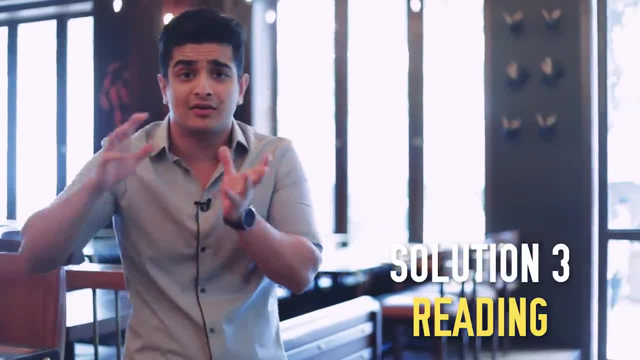 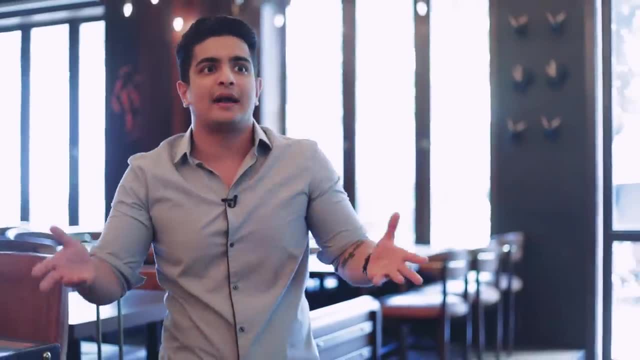 I suggest that you go and pick up an ICSE textbook, a 10th standard ICSE textbook. It's got a lot of short stories. Some people pick up a language better by reading it, so you can also go for that. You've got to figure what works for you the best. 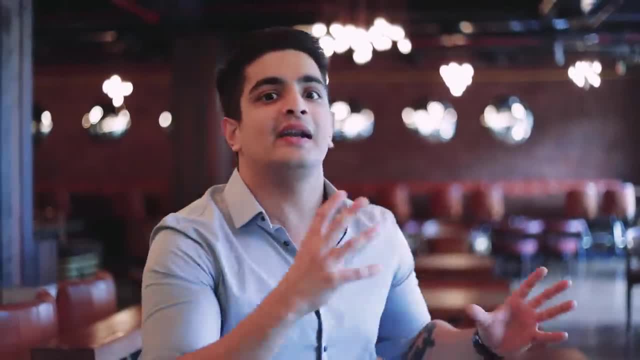 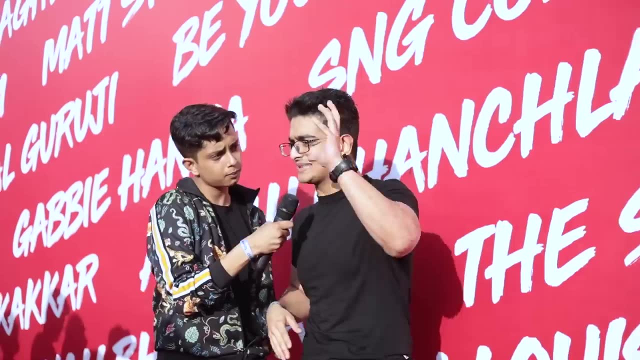 big weakness of mine. So for me to start my own Hindi channel was very difficult, But I used a few simple tricks to improve on my spoken Hindi, and I believe that those same tricks can be applied to English. As with any life skill. I believe that you've got to make the process easy for yourself. 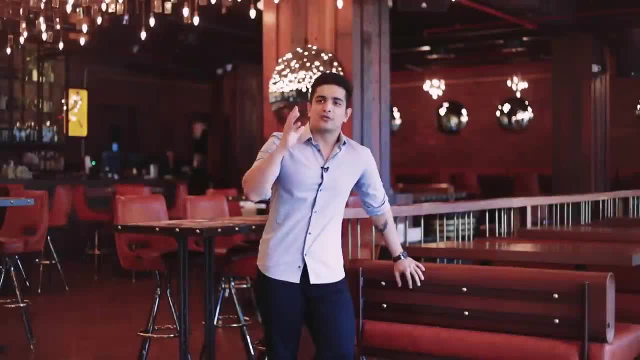 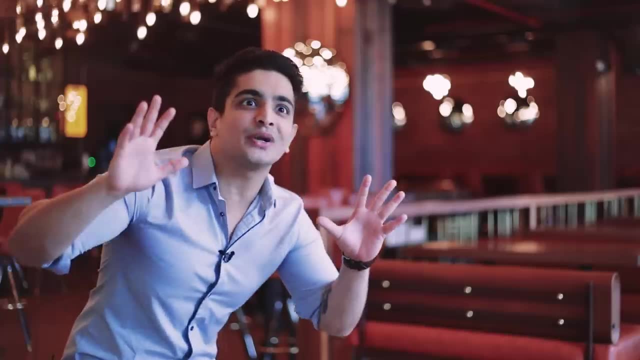 and your big brother got you covered. So if you ask most people what the first step is when it comes to improving a spoken language, they'll say: Arrey news, dekhne lag. Arrey classes, join karle Arrey. 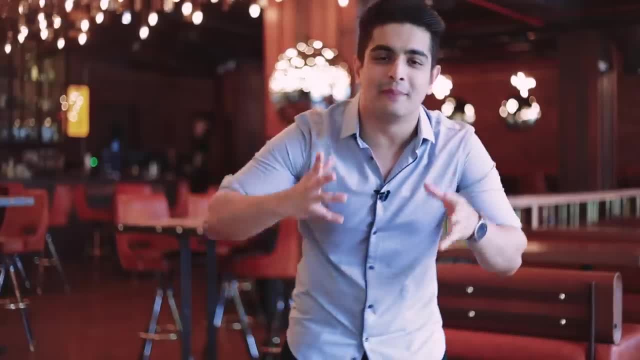 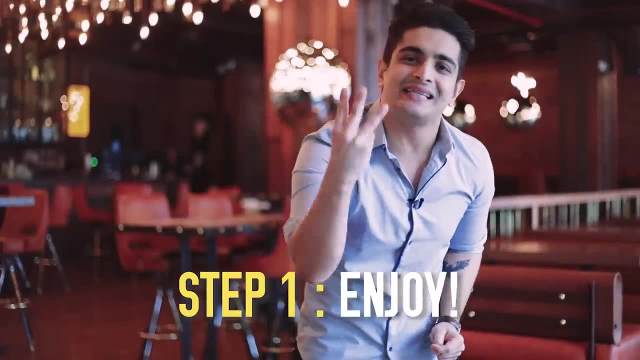 Shashi tharoor dekh bench. Nope, I don't believe that that's true. I believe that if you want to learn a new language, you've got to enjoy the process, And keeping enjoyment in mind, I've got you three easy. 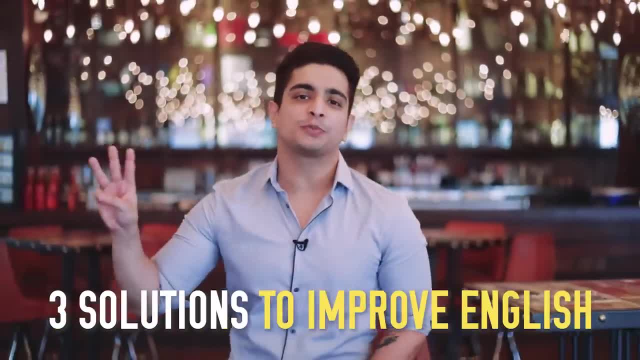 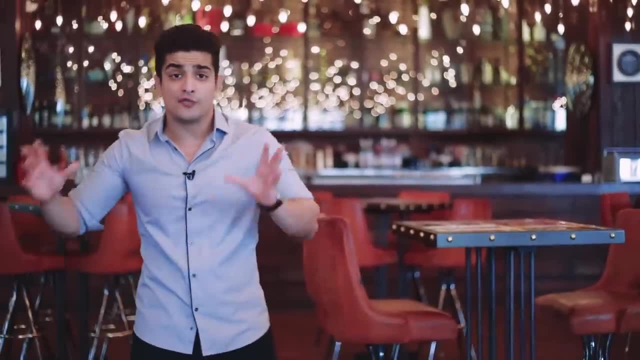 solutions. Okay, so these three solutions are basically three options in order to improve on your English. If you really want to improve it, you've got to make it a habit to practice these three options. You've got to practice it for a minimum of 15 minutes every day and for a maximum 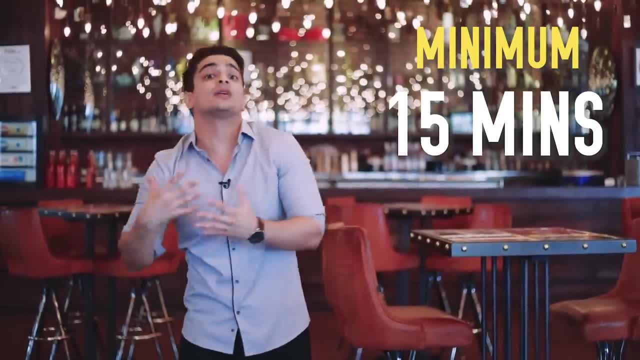 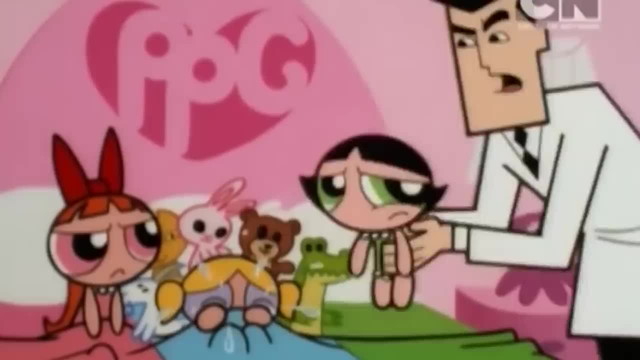 of however long you want. I'd suggest one hour a day, two hours a day. three hours a day is good. to start with Option number one, easy video content. We're talking cartoons primarily, where the language used is super simple. It's meant for children to understand. 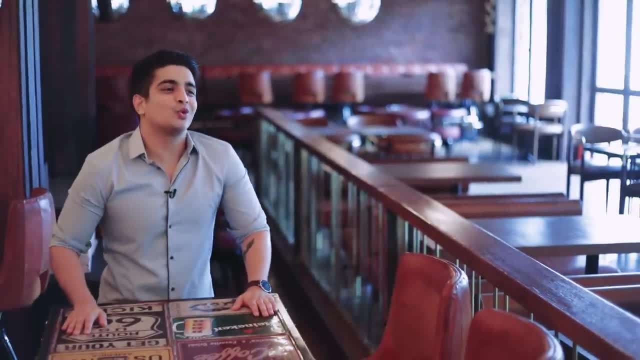 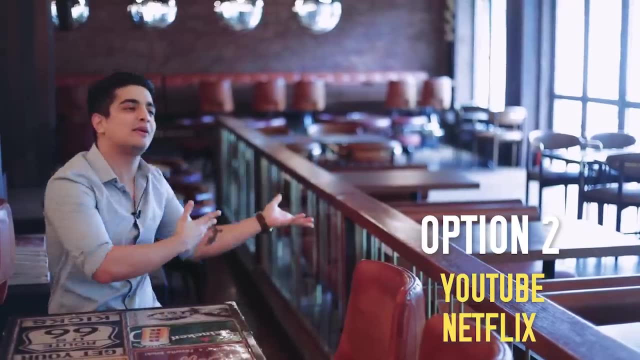 Easiest way to improve your English, And if you're one of those bros who thinks that you're too old to watch cartoons, that's okay. Your other options are to watch a lot of English video content. Maybe watch other beer biceps videos. maybe watch other YouTube channels, watch Netflix. 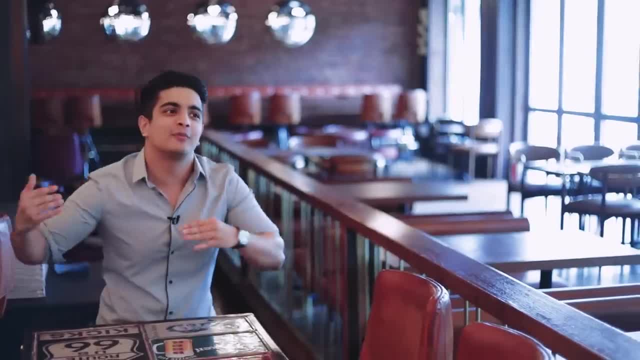 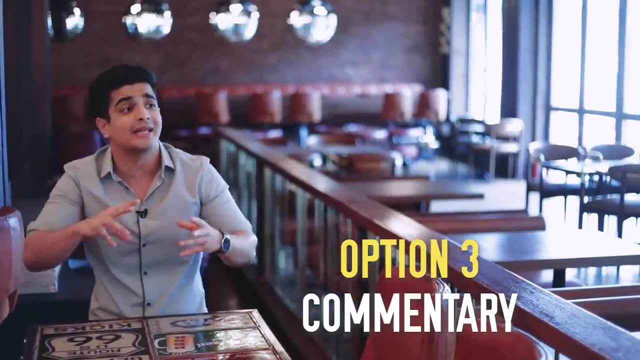 Option number three is my personal favorite. Aakash Chopra helped me to improve my Hindi by his Hindi cricket commentary Chup kar. Aakash Chopra, I'd suggest you go and watch English cricket commentary, especially Indians who are commentating in English. think Rahul Dravid, Sourav Ganguly, Harsha Bhogle is fantastic. 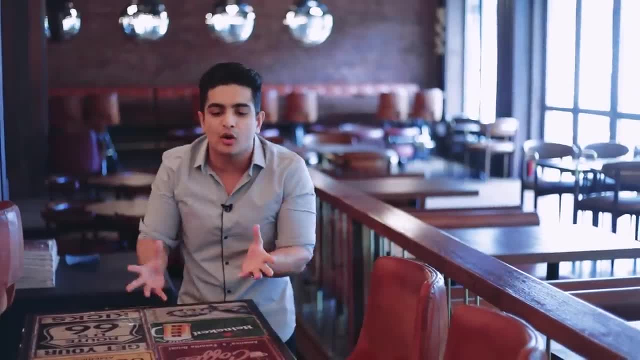 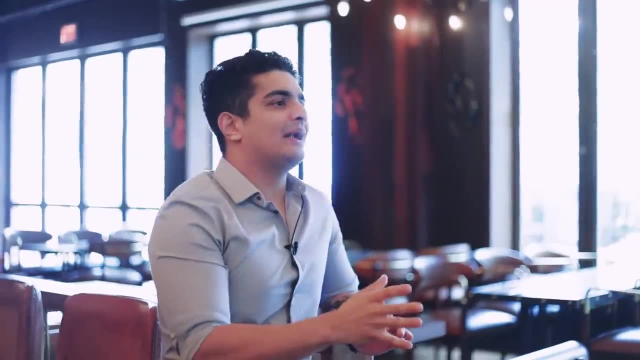 Go watch a lot of commentary. Basically, choose a piece of video content that you really enjoy watching and that'll do the trick for you. That'll help you improve on your English or your Hindi. Also, keep in mind that that's just the first solution: watching a lot of video content. 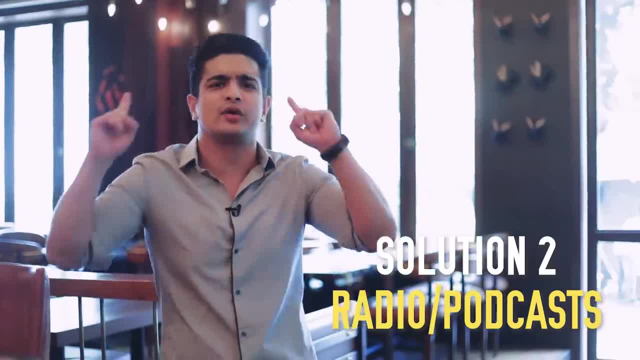 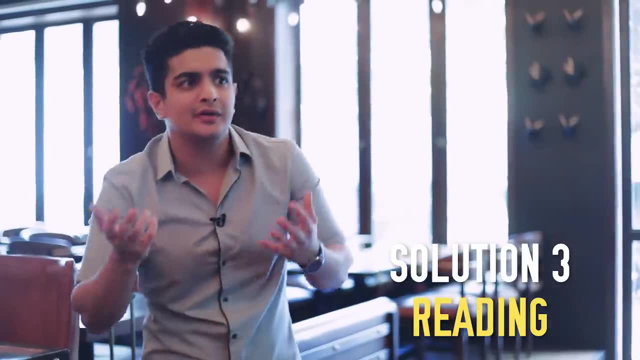 If you're someone who doesn't enjoy video content, that's okay. If you enjoy listening to the radio or podcasts, do that. And your third solution is watch a lot of Indian cricket commentary reading a little bit of simple English. I suggest that you go and pick up an ICSE. 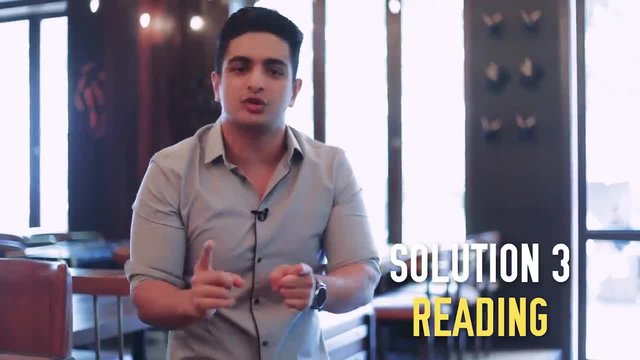 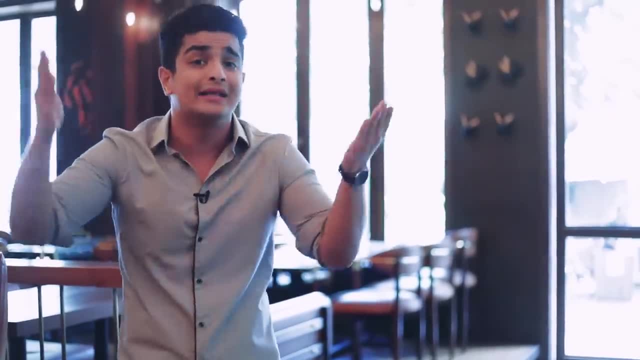 textbook, a 10 standard ICSE textbook. it's got a lot of short stories. some people pick up a language better by reading it, so you can also go for that. you've got to figure what works for you the best, what you enjoy the most and do. 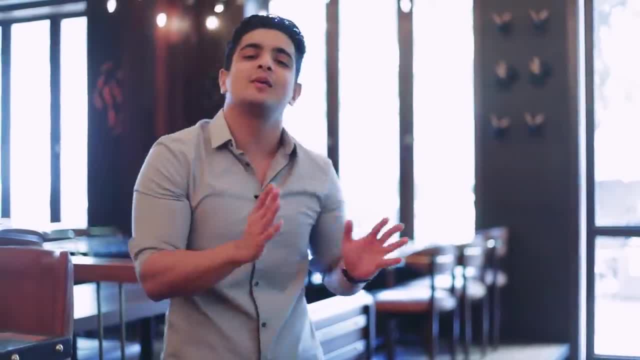 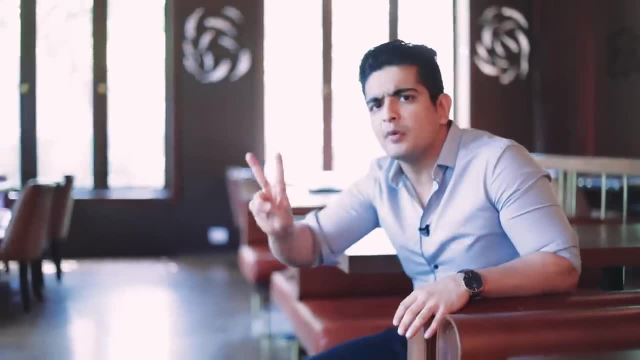 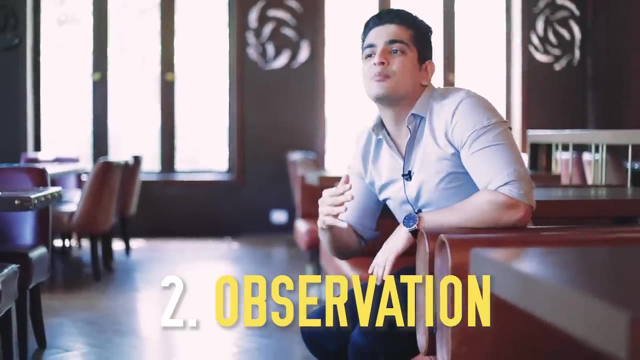 that thing every single day, minimum of 15 minutes, maximum of forever. okay, so step number one is the fun part: just 15 minutes of whatever you enjoy. step number two, once you get into a habit of practicing step number one is observing the English language from the outside. you don't have to improve your. 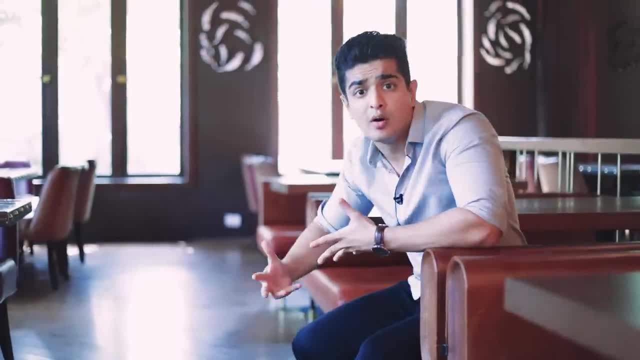 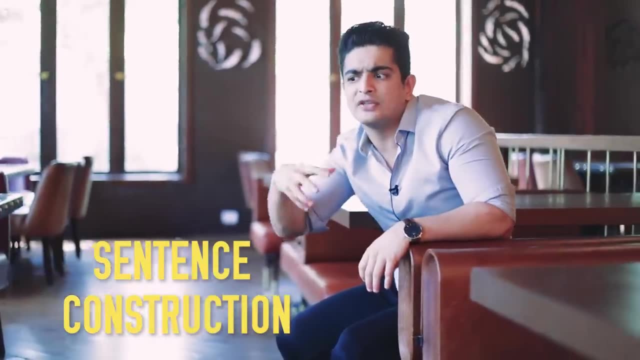 vocabulary. you don't have to learn a lot of big words. you don't have to learn new words, but what you have to focus on is sentence construction. by watching video content, you'll see that some ways in which they construct the sentences are different from the way you think. so every time you spot a difference in the 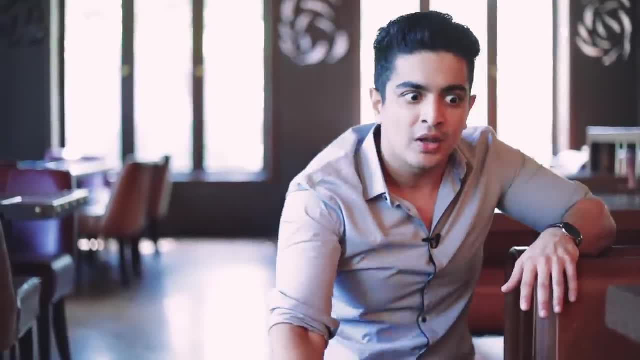 content that you're watching, or the content that you're listening to, or the content that you're reading. you've got to make a mental note of it. you've got to realize that this isn't the right way to do it, the way you speak English, and that's why your English might have a small mistake. 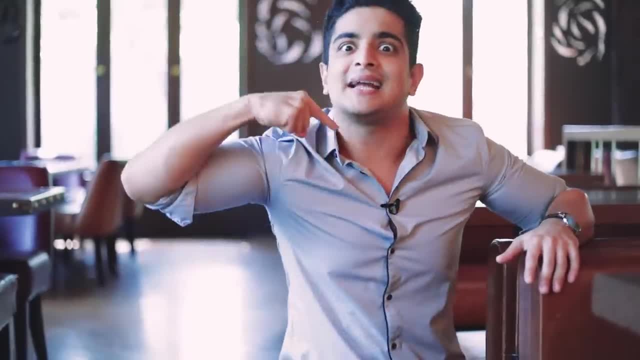 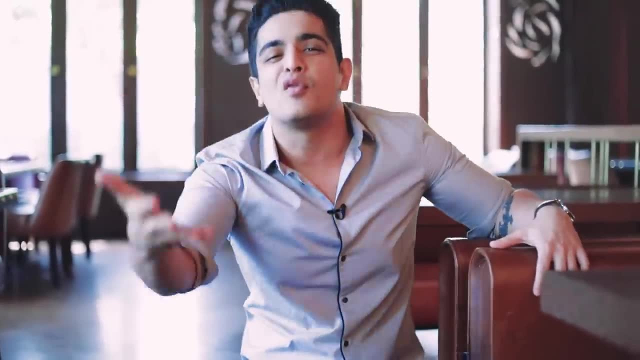 pick up on that mistake, keep it in your mind, practice it, say it ten times to yourself, just observe English from the outside. once you've figured out sentence construction, then you can think of vocabulary, then you can think of learning new words. but first understand how English is spoken and you're only 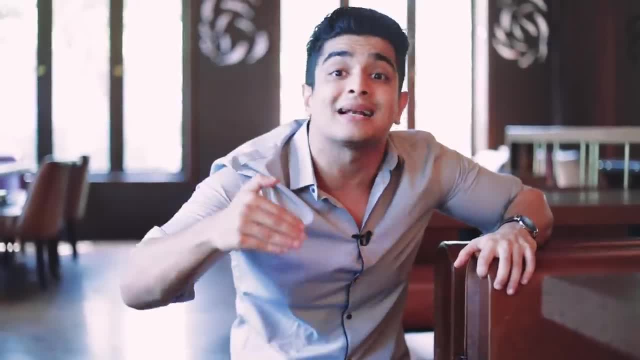 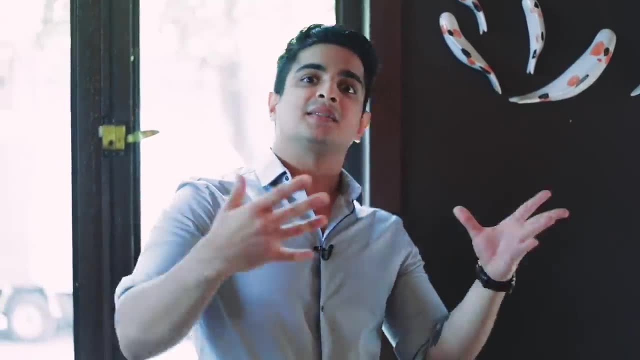 gonna have that ability to understand spoken English when you practice watching it, when you practice absorbing it into your own life. okay, step number three is not just as simple as saying: practice, karlo, it'll improve your English. step number three is about putting your ego on the side. a lot of Indians, for some reason, associate 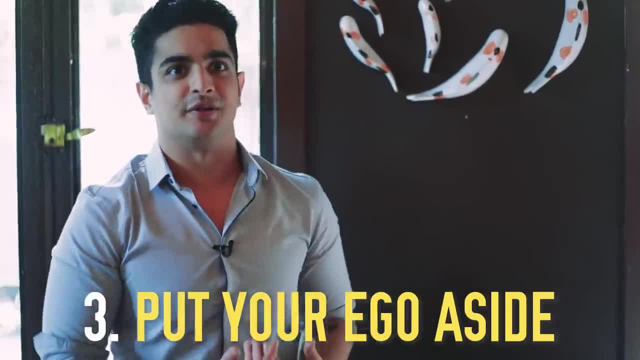 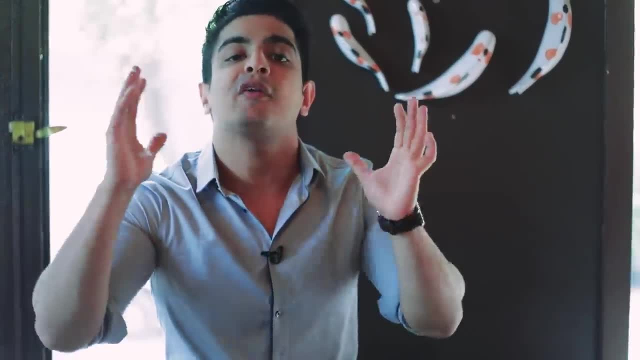 English with intelligence. if you can speak English, that means you're intelligent. so a lot of Indians actually judge other people's English very easily. but keep in mind: every time someone makes fun of you, they're not making fun of you, they're making fun of themselves, they're making fun of an insecurity. 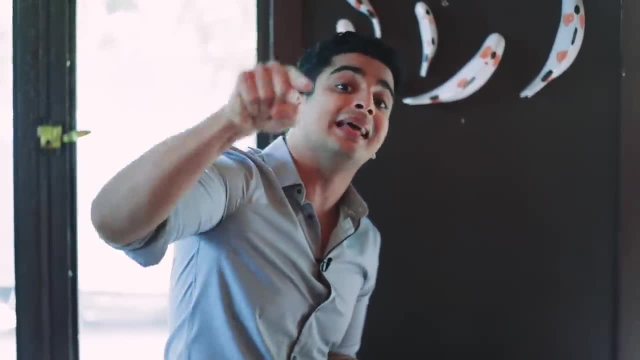 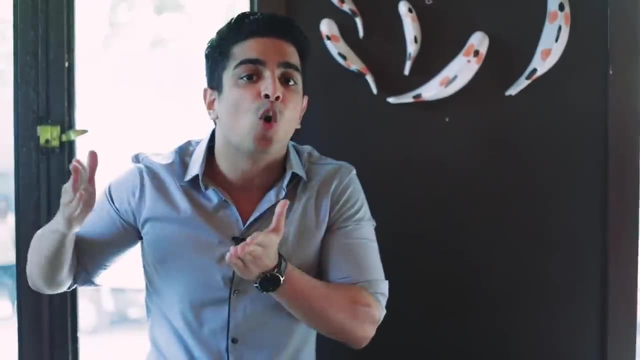 within themselves. if they make fun of your English, that means they're conscious about their own English. it's a way of boosting their own ego. that's why step number three, for me, is not about practice. practice is not about practice. it's about putting your ego on the side. you've got to get rid of your. 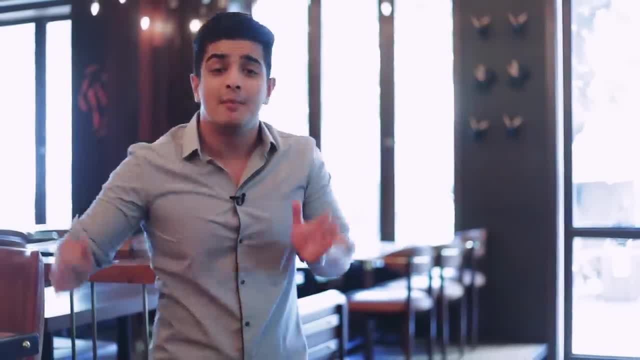 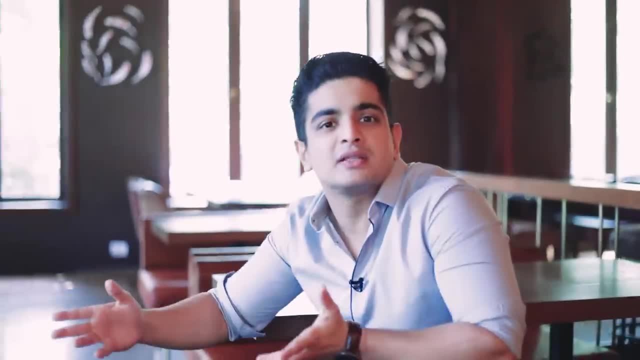 what you enjoy the most and do that thing every single day. Minimum of 15 minutes, maximum of forever. Okay, so step number one is the fun part: Just 15 minutes of whatever you enjoy. Step number two, once you get into a habit of practicing. step number one is observing. 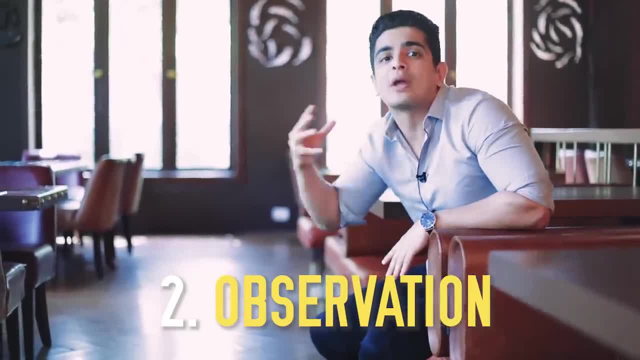 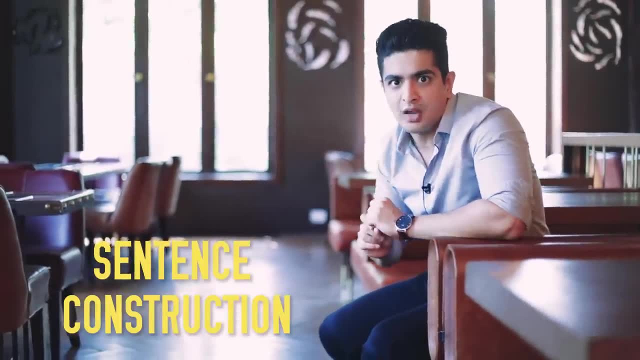 the English language from the outside. You don't have to improve your vocabulary. You don't have to learn a lot of big words, You don't have to learn new words, But what you have to focus on is sentence construction. By watching video content, you'll see that some ways in which they construct the sentences. 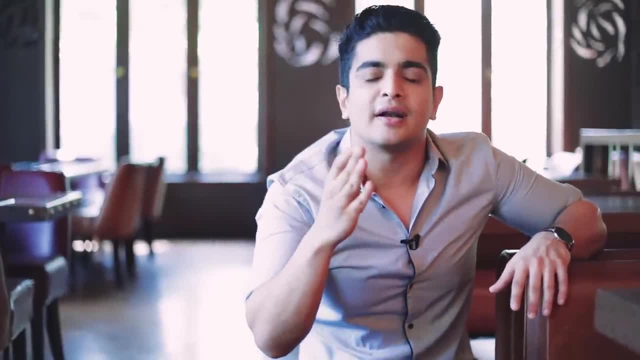 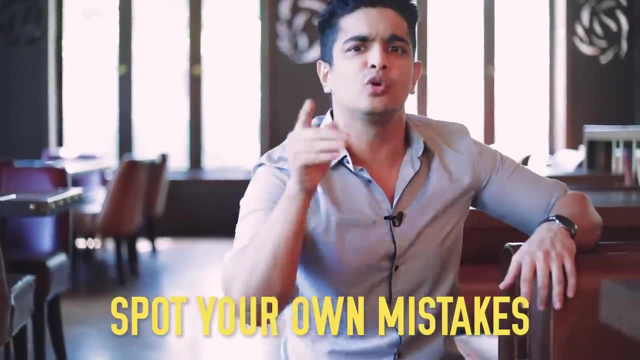 are different from the way you think. So every time you spot a difference in the content that you're watching, or the content that you're listening to, or the content that you're reading, you've got to make a mental note of it, Realize that this isn't the way you speak English and that's why your English might. 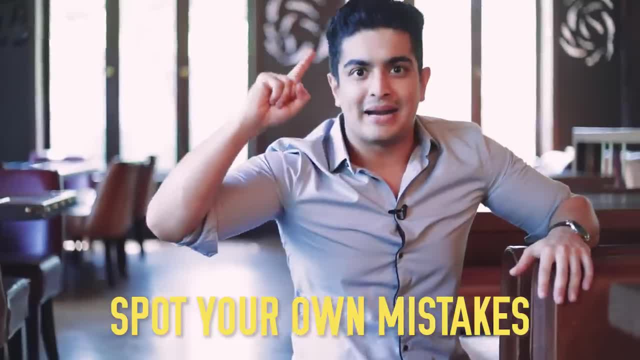 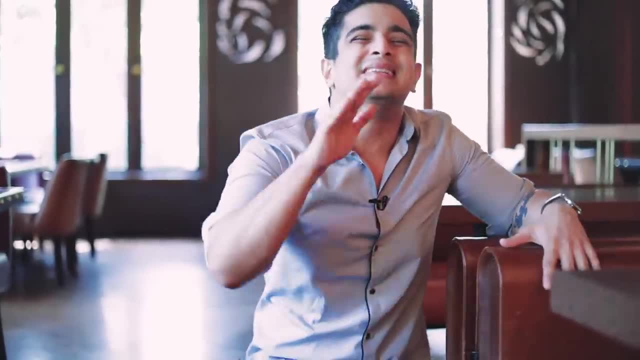 have a small mistake. Pick up on that mistake, keep it in your mind, practice it, say it 10 times to yourself. Just observe English from the outside. Once you've figured out sentence construction, then you can think of vocabulary, Then you can think of learning new words. 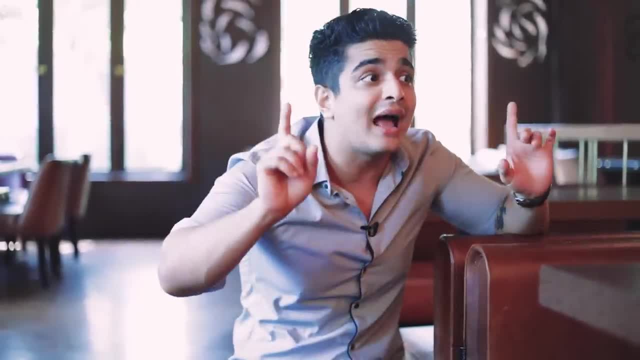 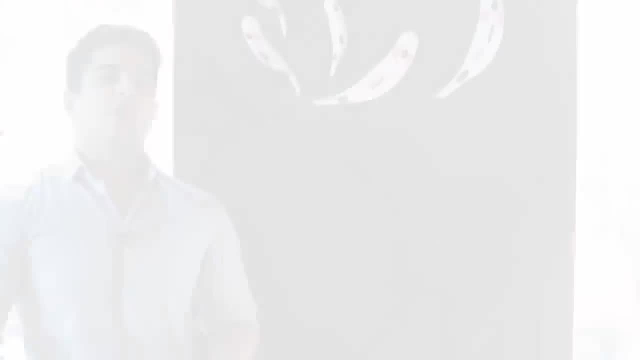 But first understand how English is spoken. and you're only going to have that ability to understand spoken English when you practice watching it, when you practice absorbing it into your own life. Step number three: It's not just as simple as saying: practice, karlo, it'll improve your English. 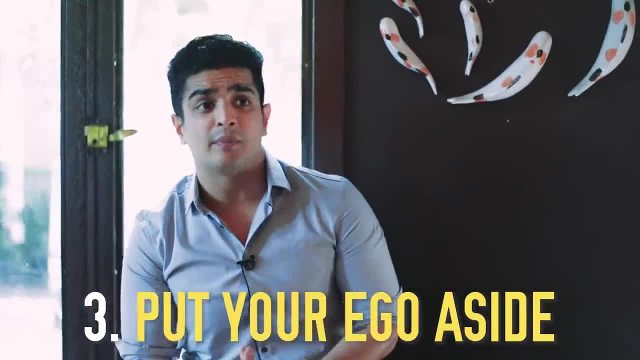 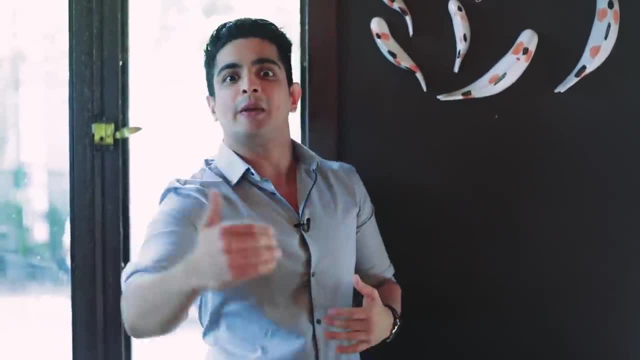 Step number three is about putting your ego on the side. A lot of Indians for some reason associate English with intelligence. If you can speak English, that means you're intelligent. So a lot of Indians actually judge other people's English very easily. But keep in mind: every time someone makes fun of you, they're not making fun of you. 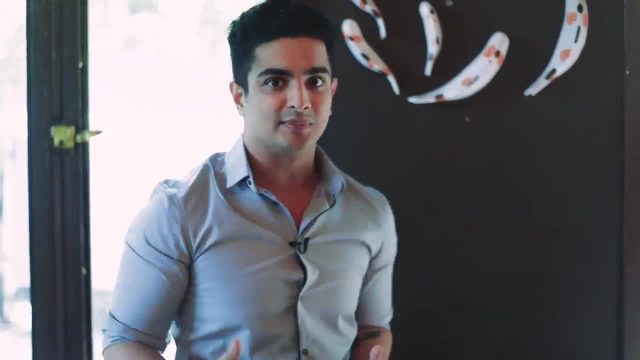 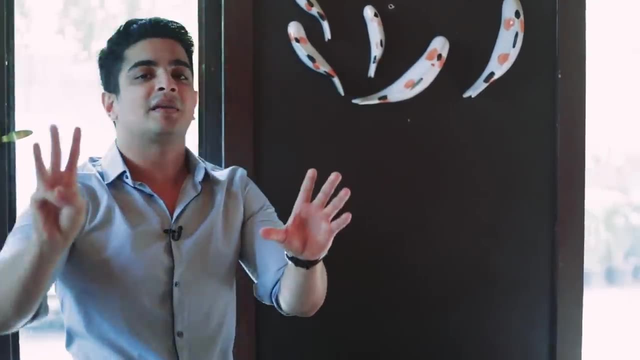 they're making fun of themselves. They're making fun of an insecurity within themselves. If they make fun of your English, that means they're conscious about their own English. It's a way of boosting their own ego. That's why Step number three, for me, is not about practice. 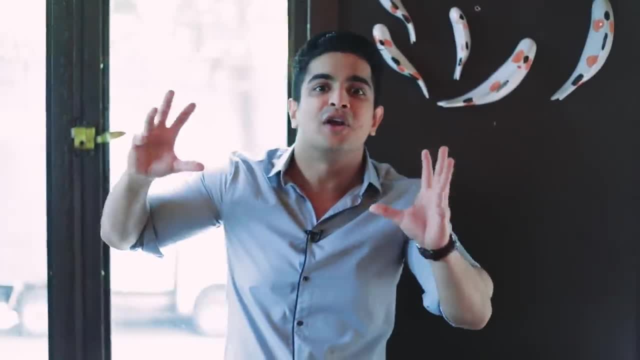 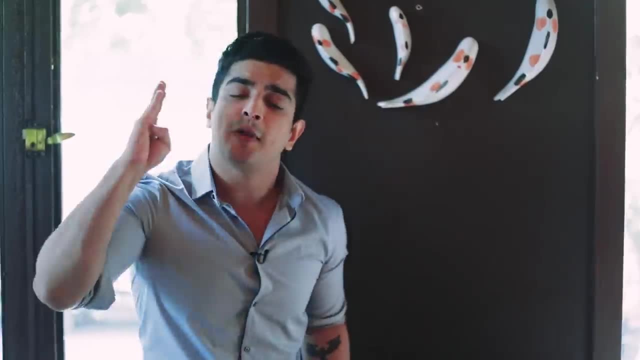 It's about putting your ego on the side. You've got to get rid of your ghamand, your arrogance Embrace mistakes. If you're speaking English and you make mistakes while speaking English, that's perfectly alright. If people point out your mistakes, you'll remember them for the rest of your life and 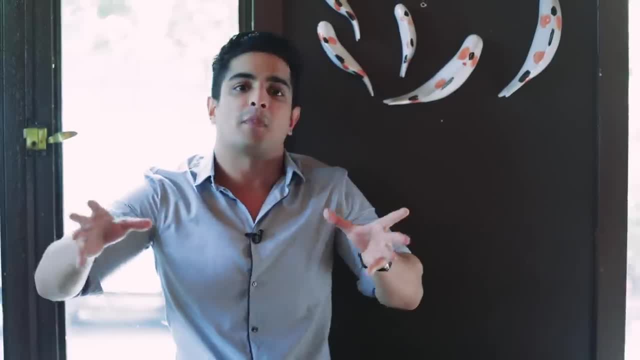 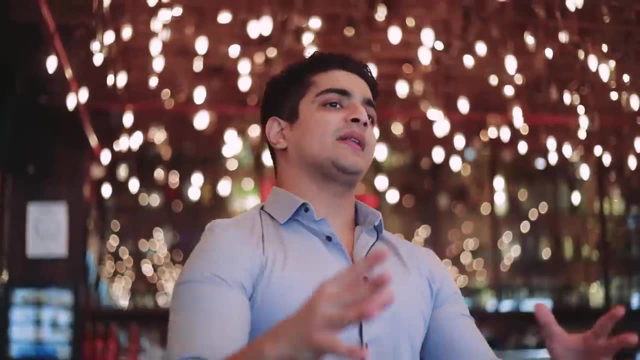 your English improves in the process. You shouldn't give a shit about what people think. You should give a shit about becoming the best version of yourself in every aspect of life. Okay, step number four, something that I learned from the world of YouTube. if you want to, 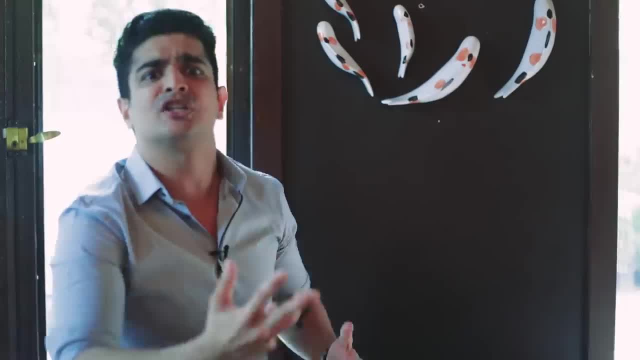 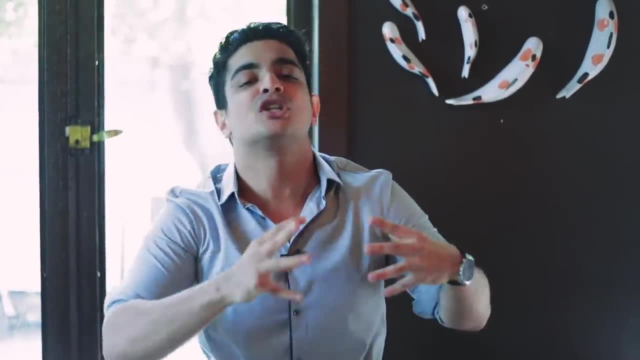 ghamand, your arrogance, embrace mistakes. if you're speaking English and you make mistakes while speaking English, that's perfectly alright. if people point out your mistakes, you'll remember them for the rest of your life and your English improves in the process. you shouldn't give a shit about what people think you. 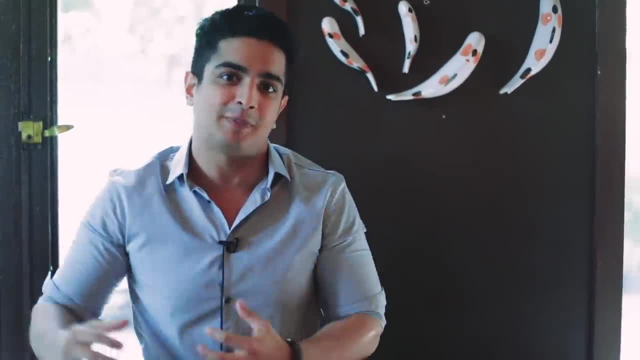 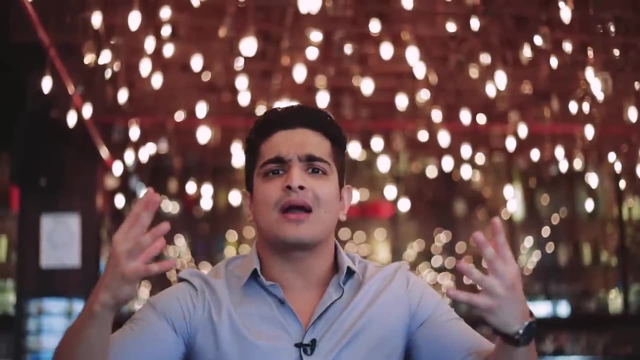 should give a shit about becoming the best version of yourself in every aspect of life. okay, step number four, something that I learned from the world of YouTube. if you want to improve any kind of spoken language, if you want to get better at public speaking, if you want to improve your communication skills, 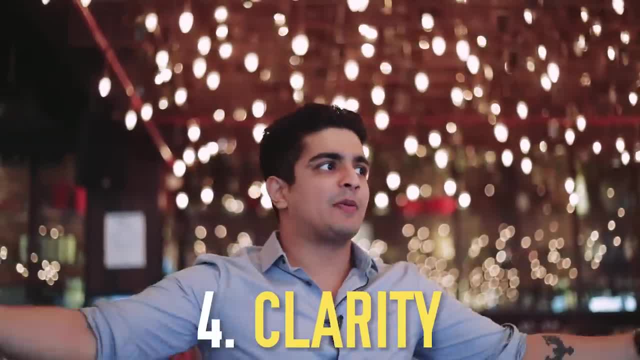 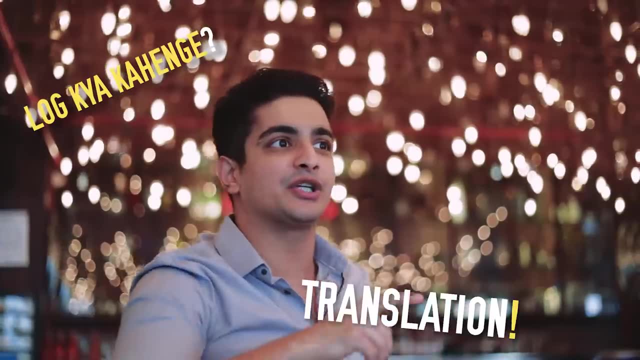 first you've got to chase clarity of thought. a lot of people are concerned about speaking English because they think of what people think, or the whole translation process from Hindi to English, or just they keep thinking of words. so clarity of thought is actually what you need to focus on to remove. 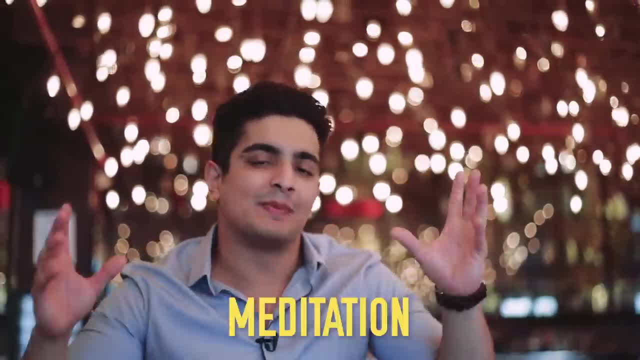 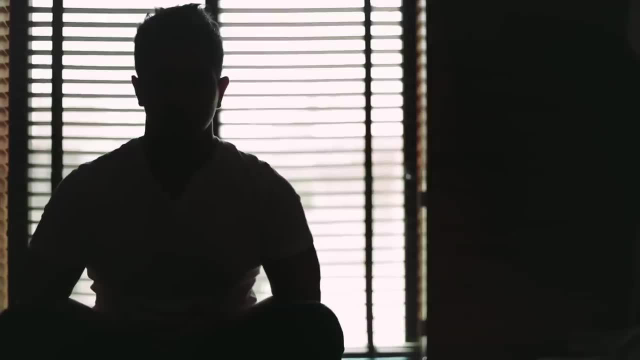 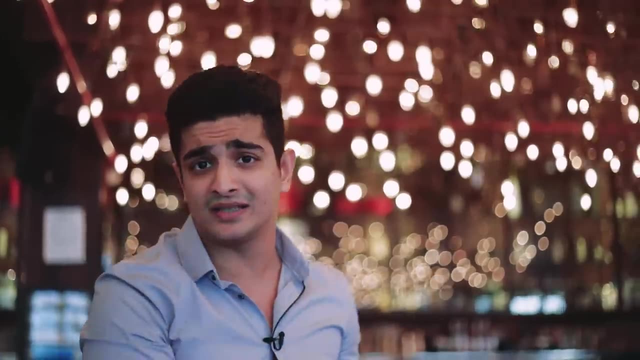 those three other bad factors. what you have to do is meditation. I know it sounds crazy that I'm bringing meditation even into this topic, but trust me, there's nothing that it clear your mind, make your thought process grounded, make your thought process clear like meditation will. if you want to know more, please watch our meditation playlist on. 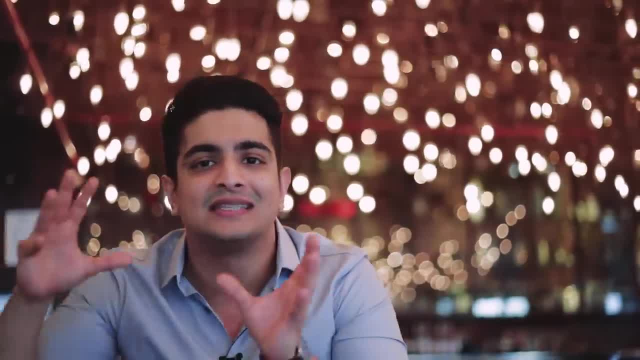 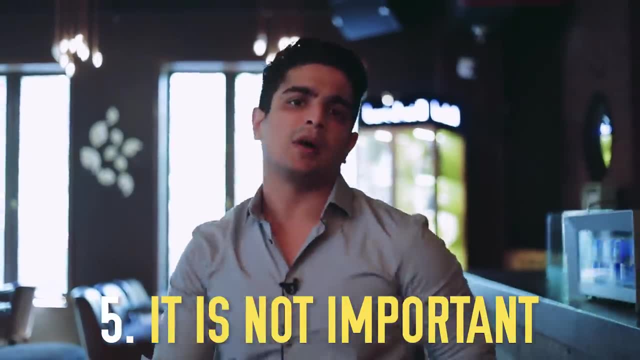 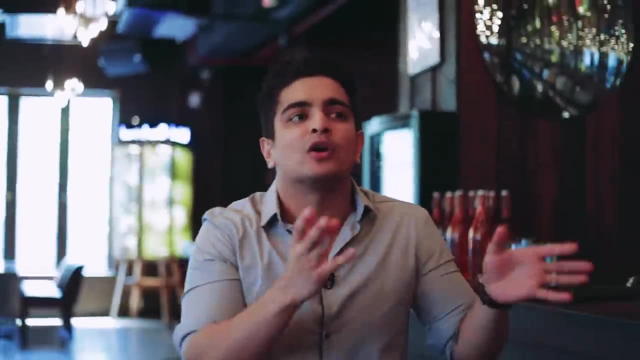 bare biceps. trust me, it'll help you with absolutely every single life skill out there. okay, fifth and final point, very simple: stop giving English that much importance. it's a huge flaw in Indian society that English is associated with intelligence, and it's a flaw because of the British. 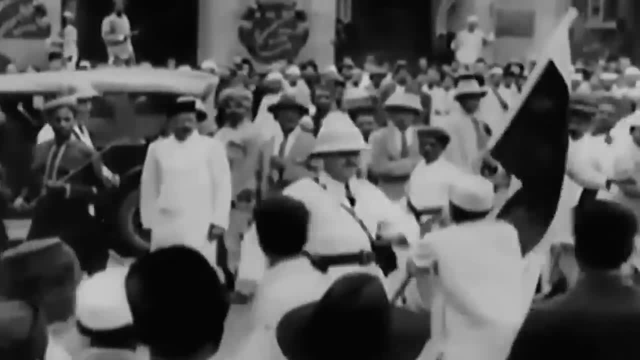 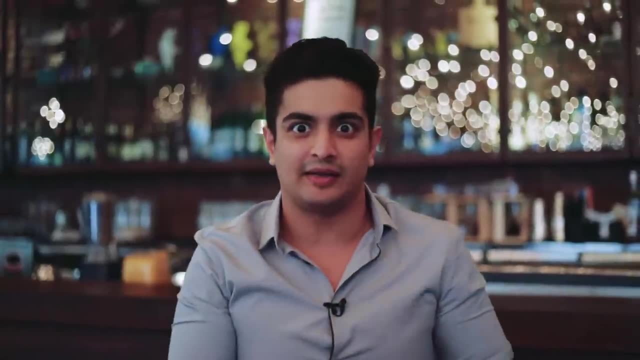 rule it 200 years of British rule- kind of put it into our heads that we should put it into our heads that English is associated with intelligence. but that's a very wrong mentality to have. nowhere else in the world will you find this mentality in Germany? people speak German. in Japan, people speak Japanese in 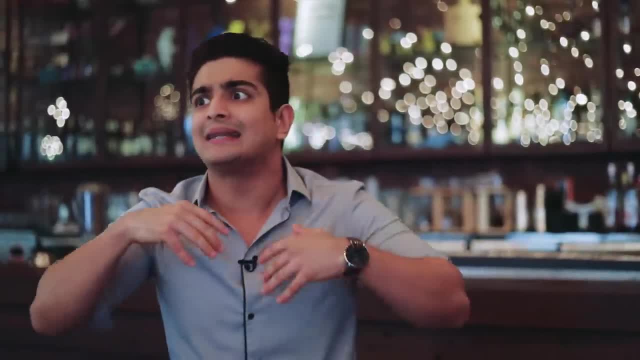 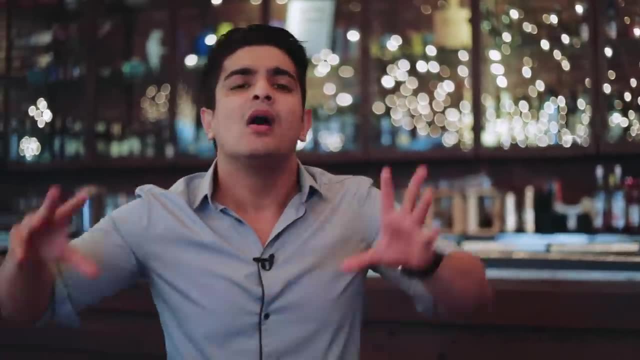 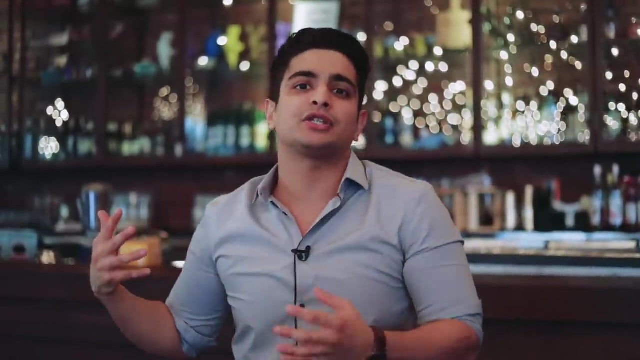 India, we should be speaking Marathi and Hindi and Tamil and Telugu and Sanskrit. that's our actual language. so I do believe that India is moving to a point in history where Hindi is okay. even while speaking English you can put in a little bit of Hindi and it's accepted. it's mostly our parents generation that. 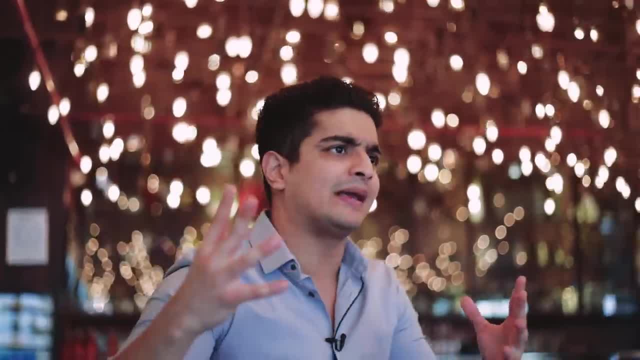 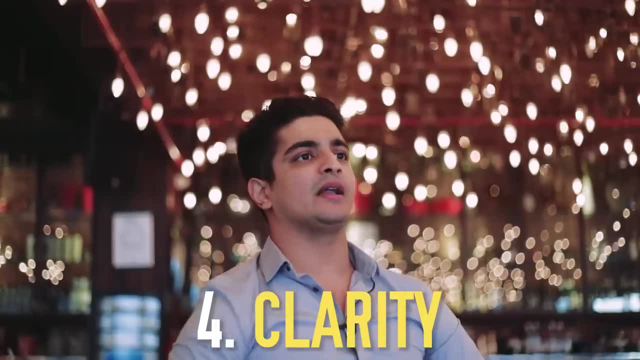 improve. If you want any kind of spoken language, if you want to get better at public speaking, if you want to improve your communication skills, first you've got to chase clarity of thought. A lot of people are concerned about speaking English because they think of what will people? 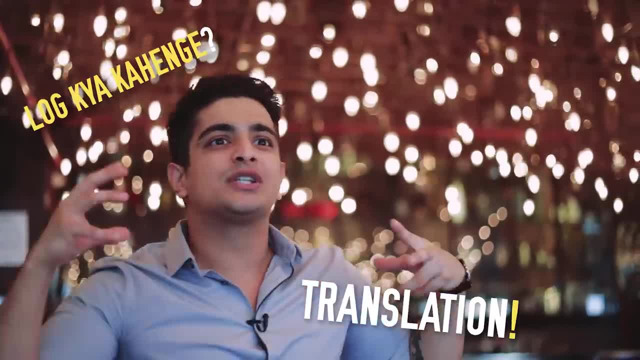 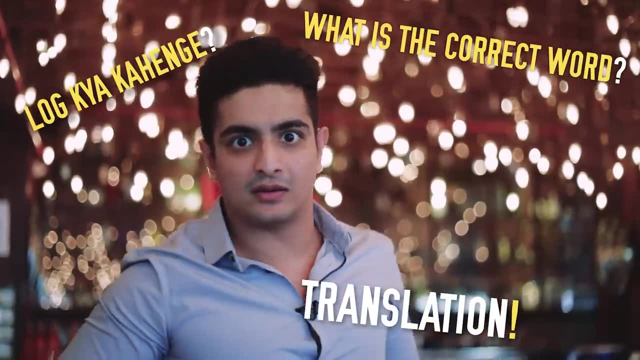 think, or the whole translation process from Hindi to English, or just they keep thinking of words. So clarity of thought is actually what you need to focus on to remove those three other bad factors. What you have to do is meditation. I know it sounds crazy that I'm bringing meditation even into this topic. 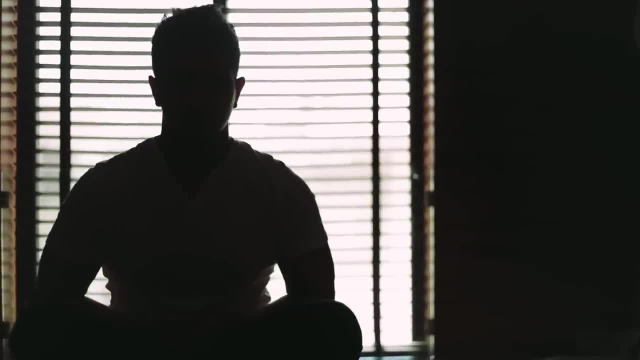 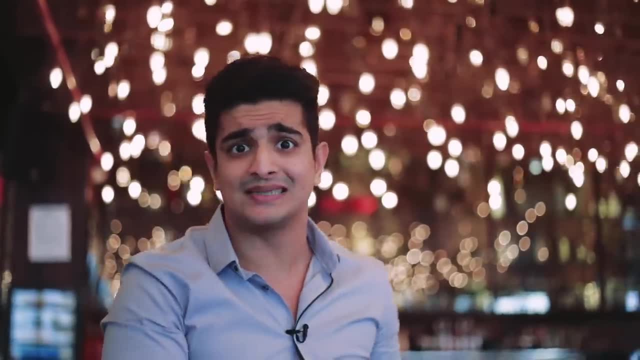 But trust me, there's nothing that will clear your mind, make your thought process grounded, make your thought process clear like meditation will. If you want to know more, please watch our meditation playlist on bare biceps. Trust me, it'll help you with absolutely every single life skill out there. 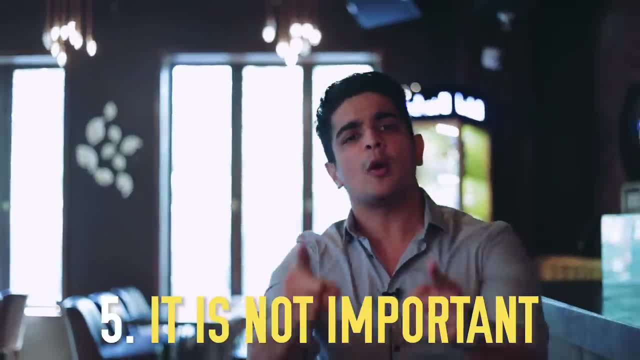 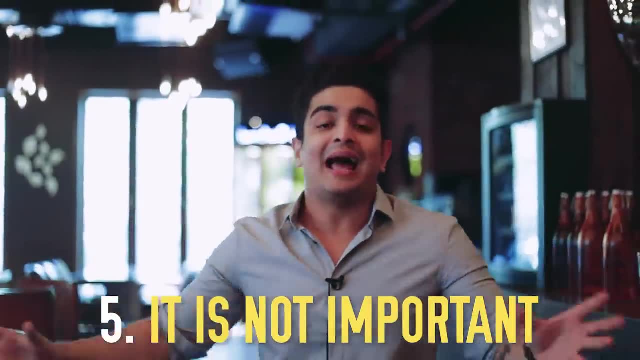 Okay, fifth and final point, very simple: Stop giving English that much importance. It's a huge flaw in Indian society that English is associated with intelligence, And it's a flaw because of the British rule. 200 years ago there was a British rule. 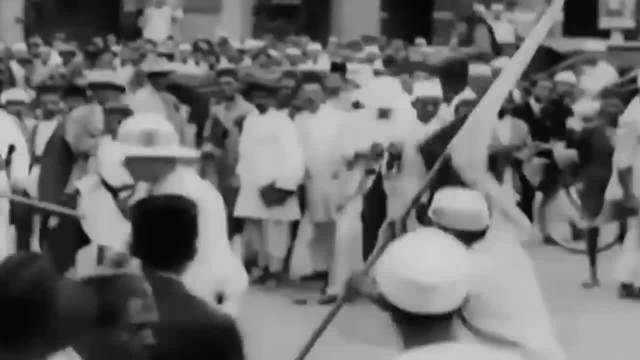 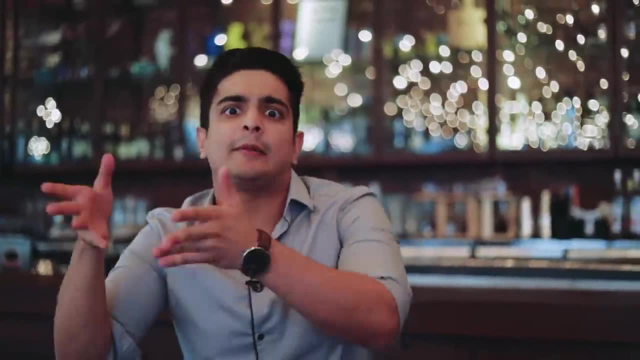 200 years of British rule kind of put it into our heads that English is associated with intelligence. but that's a very wrong mentality to have. Nowhere else in the world will you find this mentality. In Germany, people speak German. In Japan, people speak Japanese. 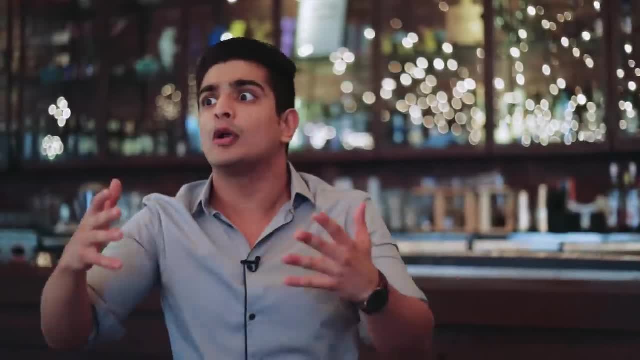 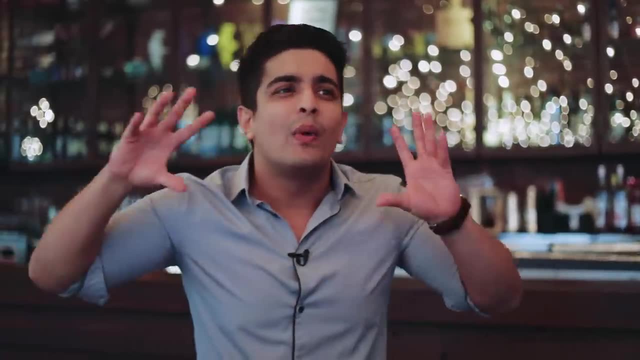 In India we should be speaking Marathi and Hindi and Tamil and Telugu and Sanskrit. That's our actual language. So I do believe that India is moving to a point in history where Hindi is okay. Even while speaking English, you can put in a little bit of Hindi and it's accepted. 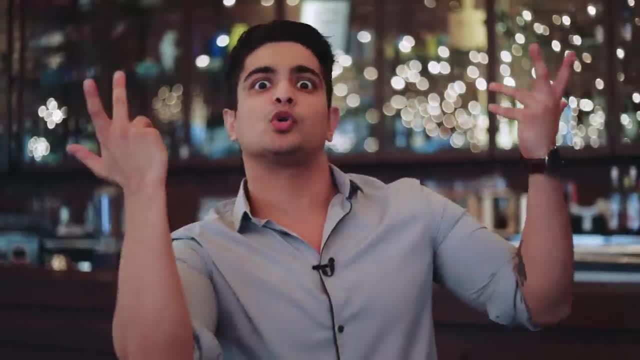 It's not like our parents' generation that thinks: Arre English bolna nahi aata aise, aise, kaise ho sakta hai? That's not the correct mentality to have. It's a foreign language. It's not from our country. 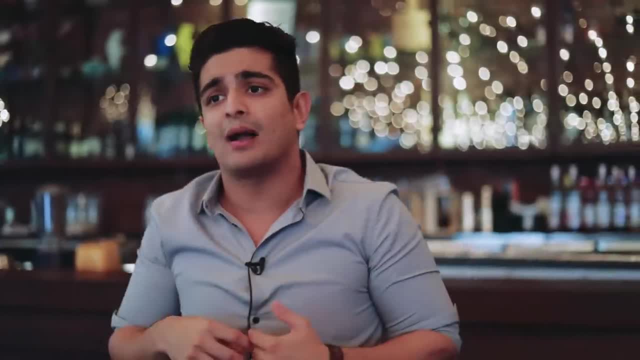 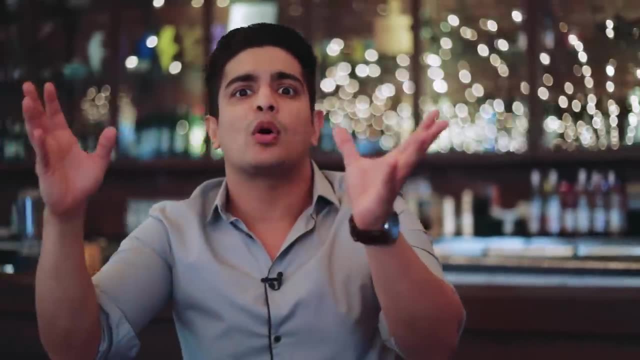 Firstly, I believe you should be proud of your own culture, your own language, And if you aren't able to speak English, well, it's really not that big a deal If you get stuck somewhere while talking English. complete your sentences in Hindi. 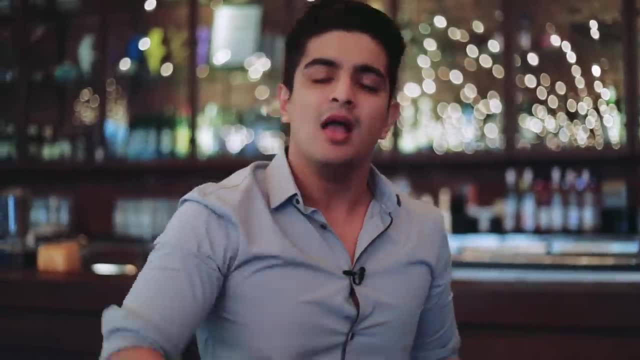 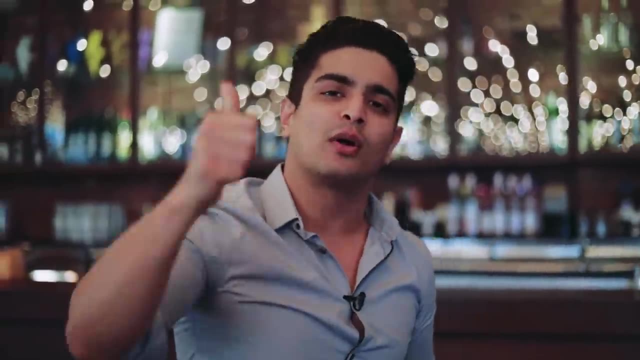 Fortunately for us, we live in an age where that is accepted. Be proud of yourself, be proud of your nation, be proud of the language that your parents and your forefathers spoke. If you enjoyed today's video, give it a thumbs up.